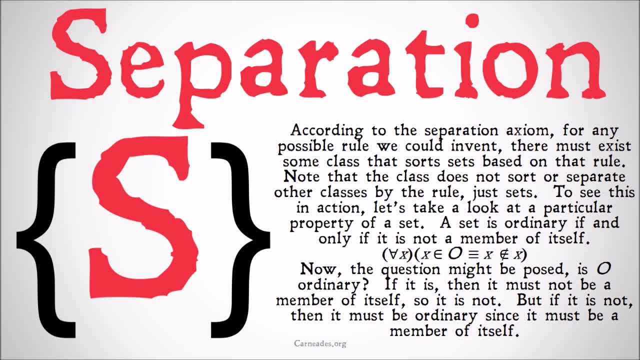 According to separation axiom, for any possible rule we could invent, there must exist some class which sorts sets based on that rule is a simple way of saying what happened to the last video. last video is pretty complicated. basically we're saying that for any rule, there has to be some class which 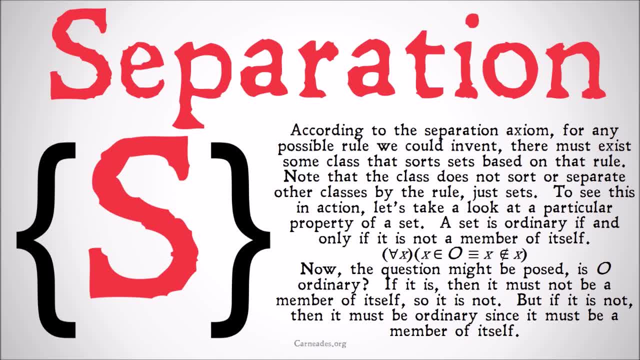 says: sets that are members of this class follow the rule. things that are outside of this class don't follow the rule. note that the class does not sort or separate other classes by the rule- and this is very important- just sets, remember i mentioned in the last video. there's a difference. 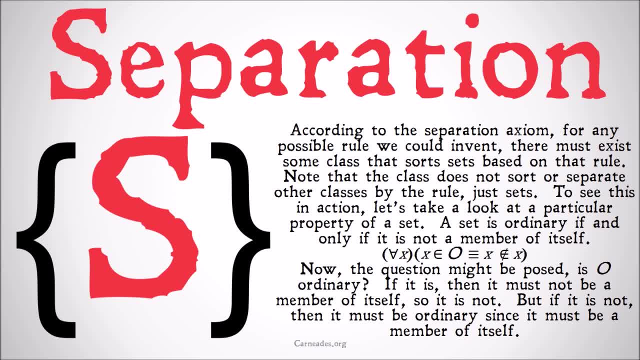 between those capital a and b and the lowercase x. the lowercase x is talking about sets, the a and the b are talking about classes. this is really only time, the only time that the distinction between classes and sets is going to matter in such a big, important way, at least for now. 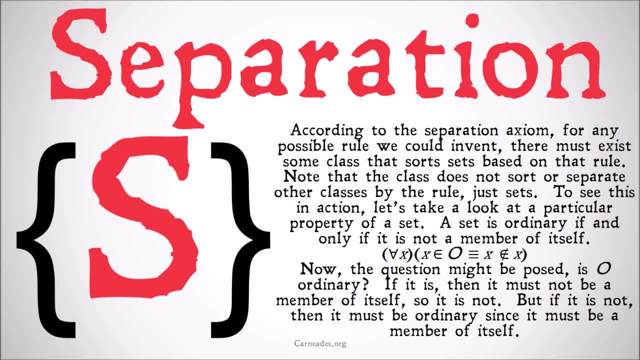 so we're saying that the class can pick out a set of sets, a class of sets which follow a certain rule, but they can't pick out a set of classes or a class of classes that follow a certain rule. why? because of ordinary things. so there's a particular property of set called an ordinary set. 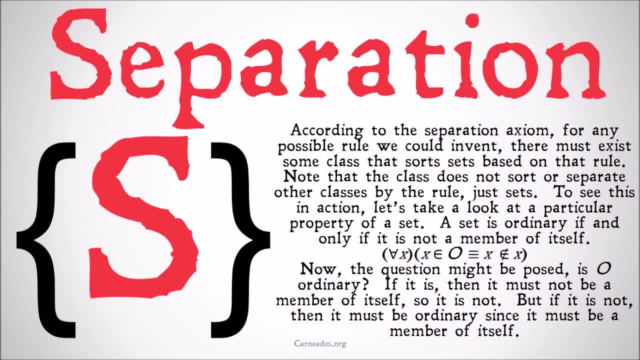 a set is ordinary if, and only if, it is not a member of itself. for all x. x is a member of o, so o is a class of all ordinary sets if, and only if, x is not a member of x. so this seems like a fairly intuitive property we want to be able to split. 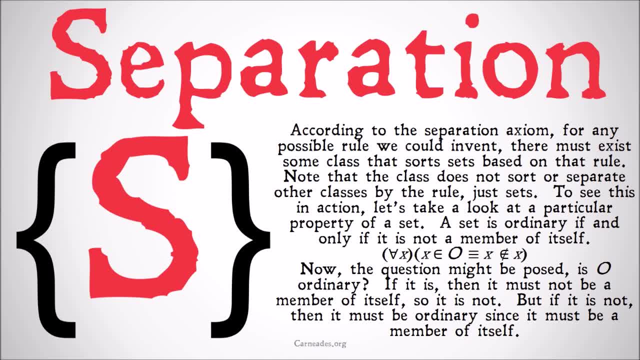 sets into the sets which are members of themselves and the sets which are not members of themselves, and you think you'd be should be able to do that right. it seems like an intuitive property. we could frame it in terms of the axiom of separation, but also it seems sensible, it seems intuitive that 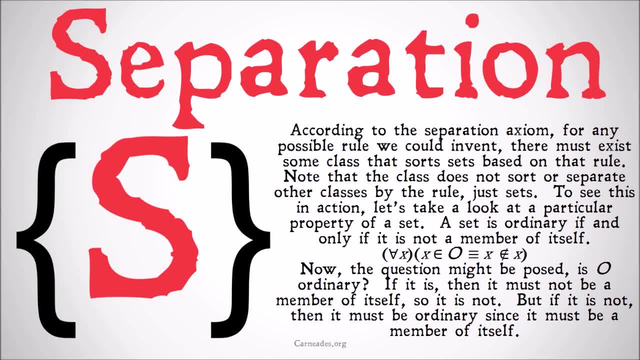 we want to be able to separate out sets that are members of themselves and sets that aren't. the question might be posed now: is o ordinary, this class that we've created, which is the set of the class of all sets which are not members of themselves, is it a member of itself or not? 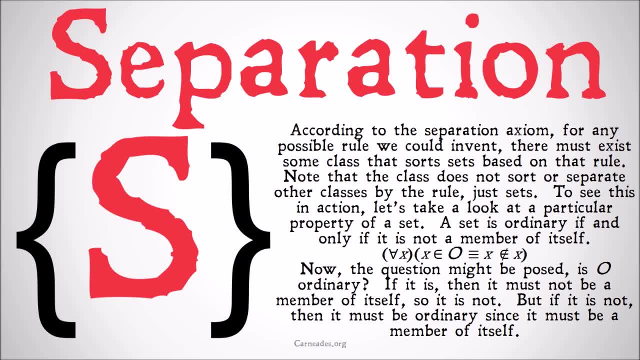 if it is a member of itself and o is a set, then it can't be a member of itself because it doesn't pass the criteria, because it's not not a member of itself. but if it's not a member of itself, then it must be a member of itself because that's the definition of being ordinary. 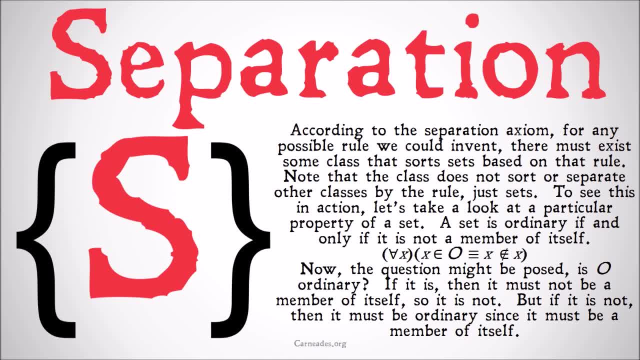 the only recourse we have is to say that such a set does not exist, but that causes problems for our axiom of separation. if such a set doesn't exist, unless we have the distinction between sets and classes, what we can conclude is that o can't be a set because o can neither be a member. 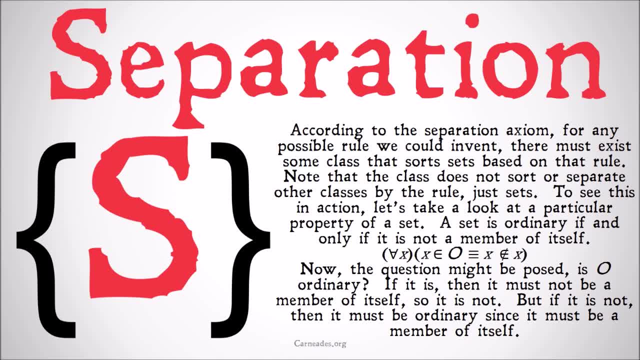 of itself, nor not a member of itself. it must not be the kind of thing we're talking about. it must not be a set, it has to be something beyond sets, it has to be a class. so o then can't divide out all classes into things that are ordinary or not ordinary, because 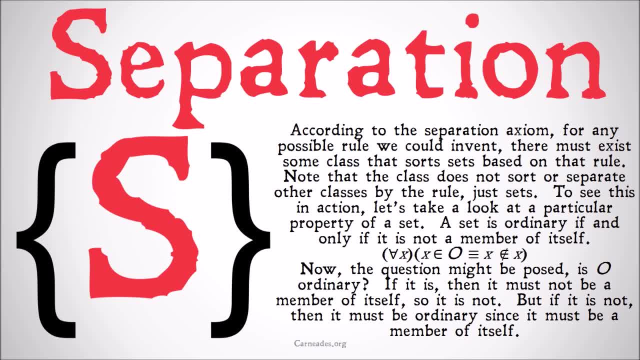 then it would be required to make a decision about itself and it's impossible to make a decision about where O falls. But if O as a class makes a distinction about sets, then it's possible because O can make a distinction about all of the sets because it's not a set itself. 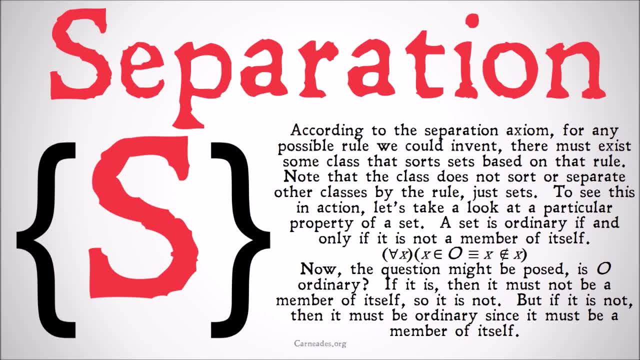 That was complicated. Check out my videos on Russell's Paradox, as well as Zerbello-Fraenkel set theory If you want more context for this. we'll dig into it a little bit more in the next couple of videos, but that's what's going on here. 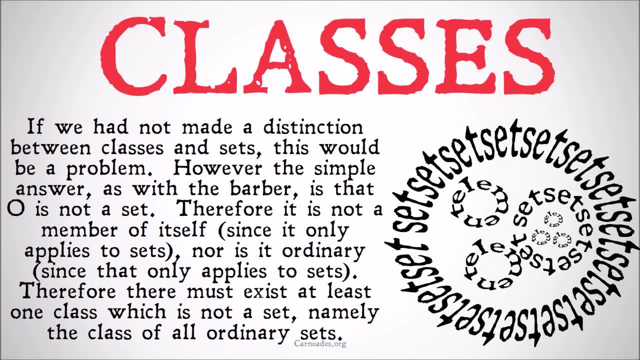 If we had not made a distinction between classes and sets, this would be a problem. However, the simple answer, as with the bar verb, is that O is not a set. O is a class. Therefore, it is not a member of itself, since it only applies to sets. 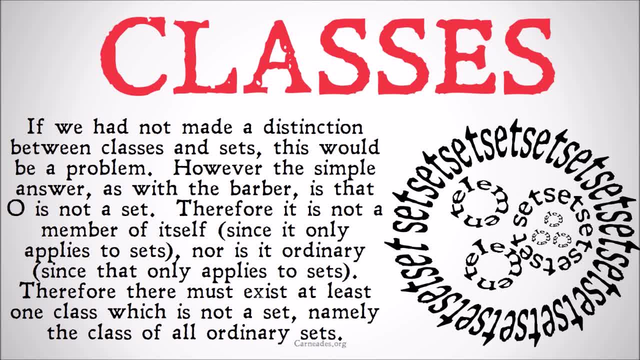 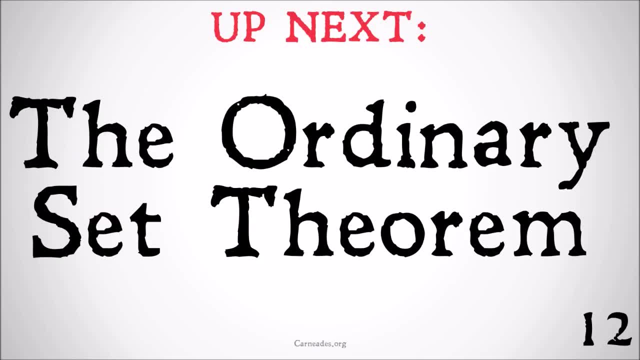 Nor is it ordinary, since that only applies to sets. Therefore, there must exist a set, There must exist at least one class which is not a set, namely the class of all ordinary sets Up. next, to continue on this. like I said, we're going to keep drilling down on this.